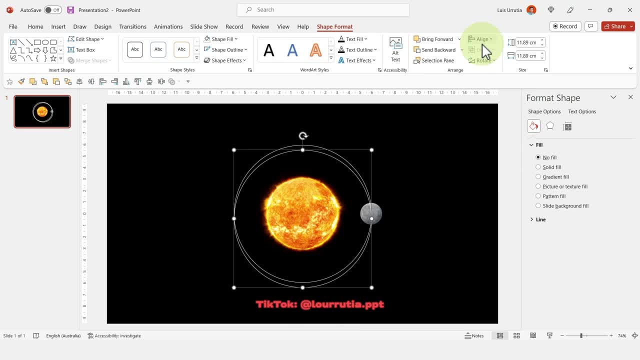 of the orbit. So you select the orbit- ctrl-c, ctrl-v- and then align it to center and middle and holding shift on your keyboard you can go to thegoing image function, away from the chalk. You can edit this to what you like. you can want a empty space, you can put in the cane and peace, the fog, but you can also save it. you can input some inner details in there as a comment, or you can enter next to your files. 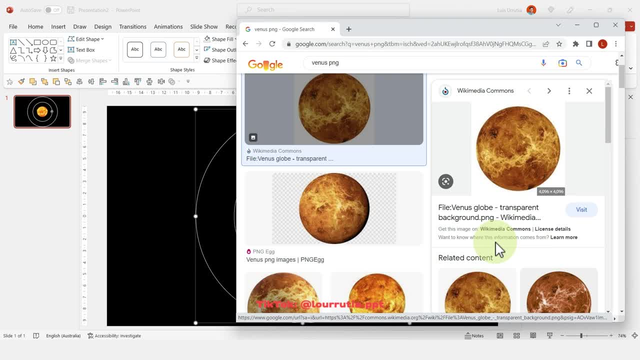 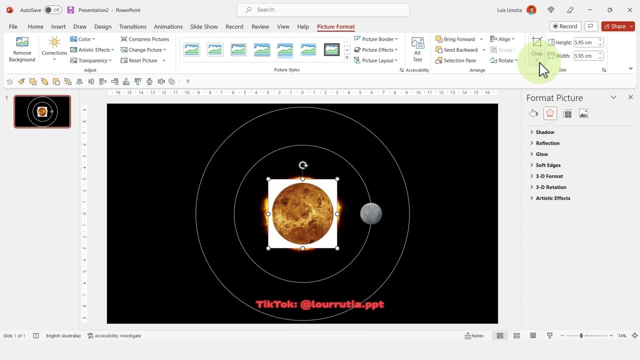 on your keyboard you can make it larger. and again I'm gonna insert an image of the planet, which in this case is Venus. and another method to get rid of the white background is you go to crop, crop to shape and select the circle here, then click on crop again and just make the image a little bit larger and that's. 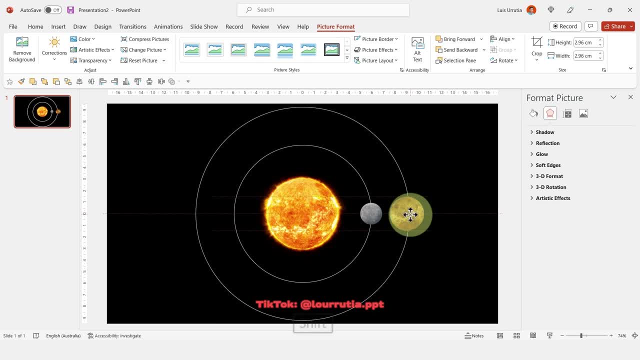 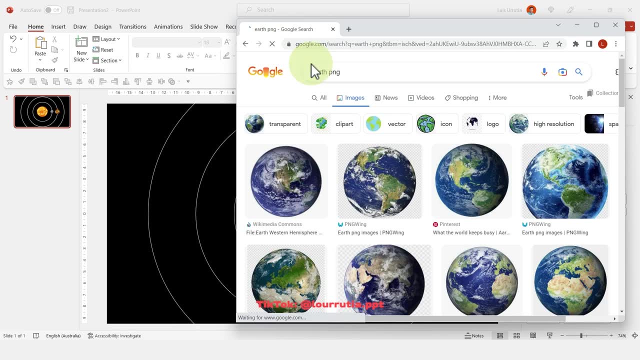 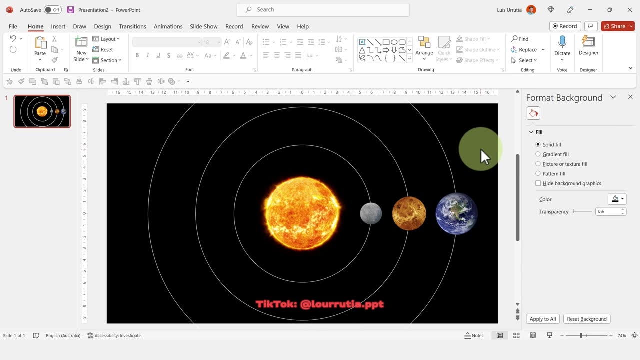 just another way to get rid of the background, and I just repeated the process with making the duplicates, and then I added a third orbit where, in this case, I'm gonna put the earth again, create the duplicate, make it transparent and group it. now you're gonna select the three groups and then go to animations. 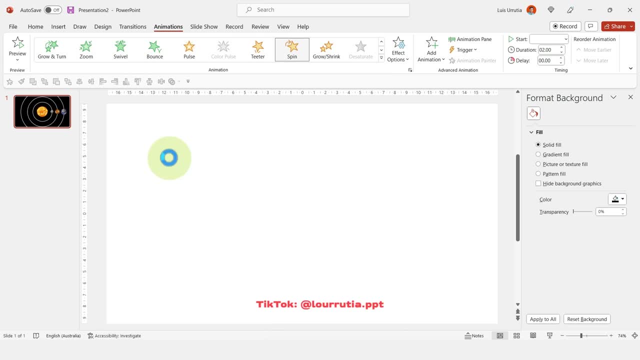 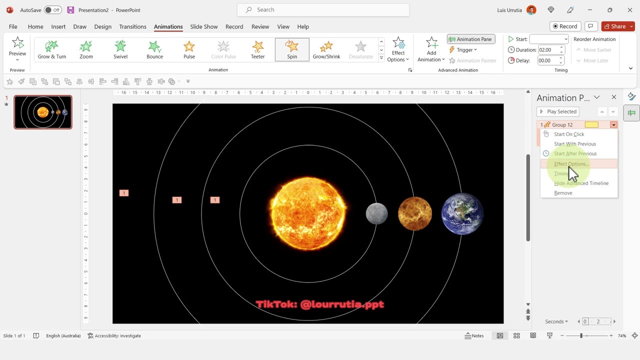 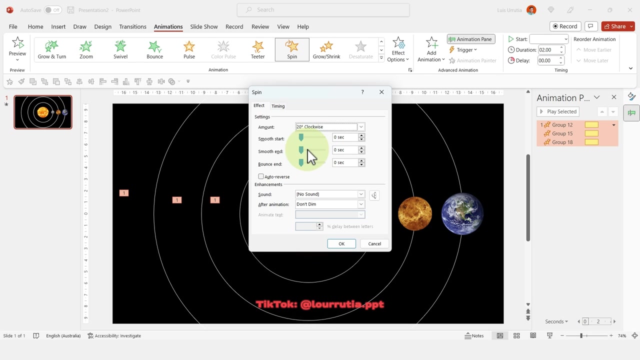 and click on spin and it's gonna look a little wild at the moment, but we're gonna fix that in a second. so you just have to go to animation pane, right click effect, object options and here we're gonna change: instead of 360, we're gonna change to 20. 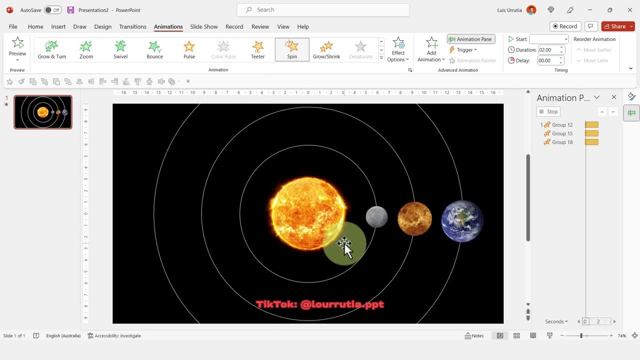 degrees and just smooth the end to 2 seconds and click OK, and then we're gonna select Venus, which in this case is this group right here. so right-click effect options, and here we're gonna change from clockwise to counter clockwise, and then, to make it a little bit more dynamic, I'm just gonna rotate. 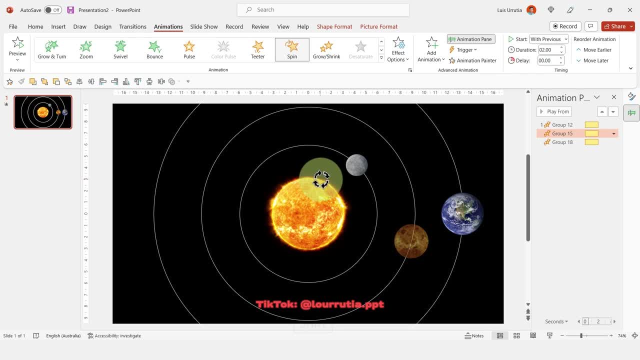 these planets here and then I'm just gonna rotate them and then I'm gonna divide them into two parts so that they have a little space here, so that they don't see it on the same kind of like horizontal line. so now it's looking a little bit more dynamic, to add the glowing effect to the planet you just 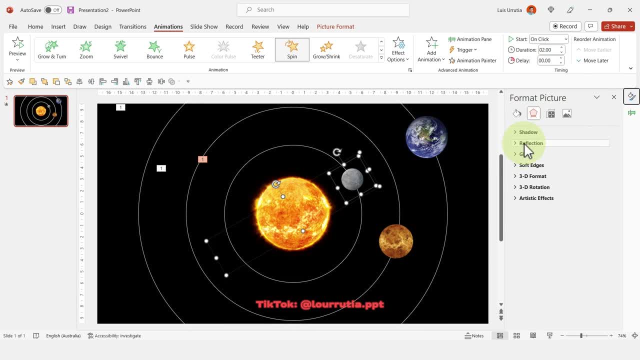 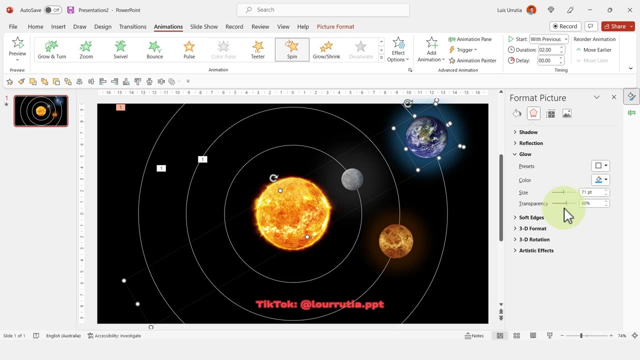 have to select the planet, go to format picture, click on glow and here you can select preset. so then you can just increase the size and change the transparency, and once you're happy with how your glows are looking- the little looking- just have to zoom out, select everything and make it larger. holding: 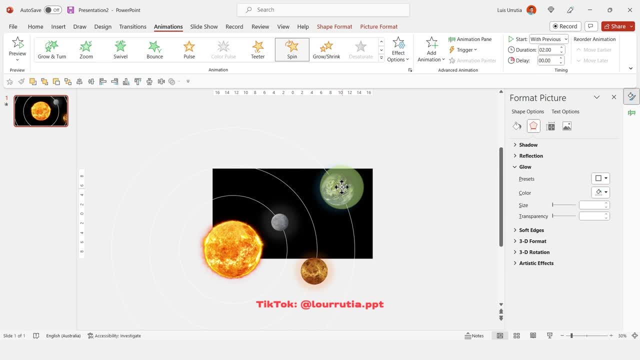 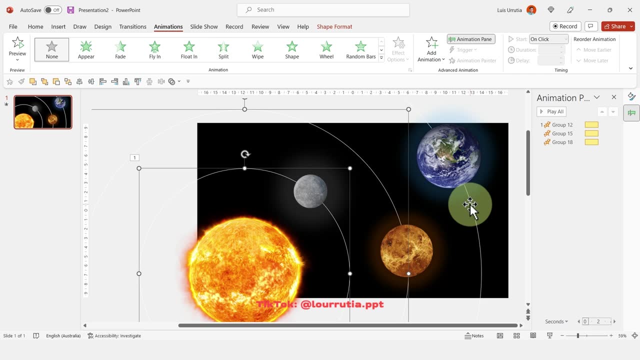 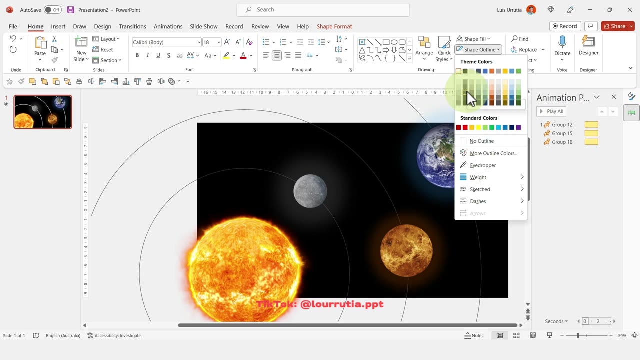 shift in your keyboard and then you can just move it. so the Sun sits on the left bottom corner, and then I'm gonna fade the orbits a little bit, because I think that the white is very, it's very bright, so I'm just gonna change it to to a 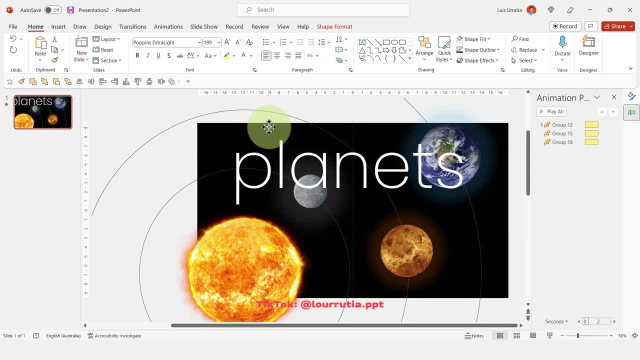 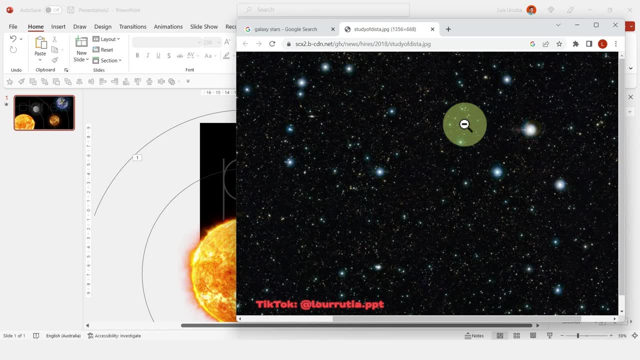 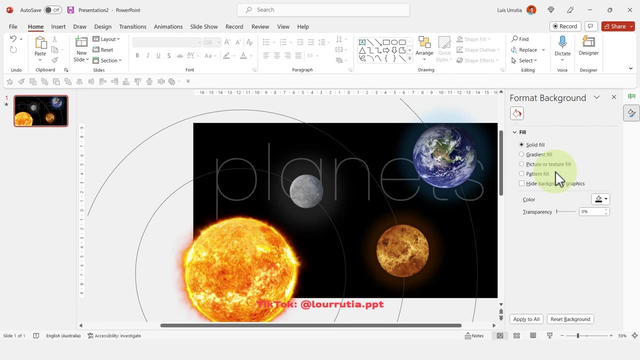 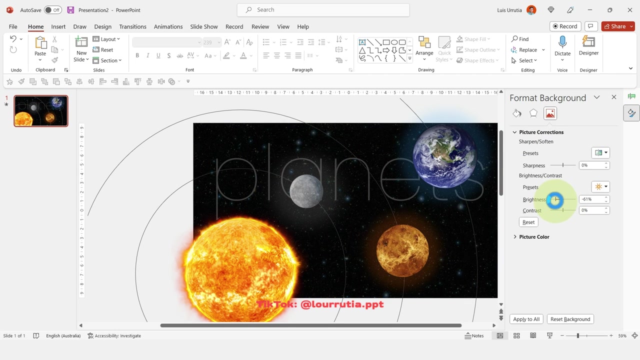 light gray and then I just added my text and right click send to back and I changed the color to gray, then I added a galaxy background. so right click copy and then right click format background and here you can select a picture or texture field and then click on picture corrections and decrease the brightness. 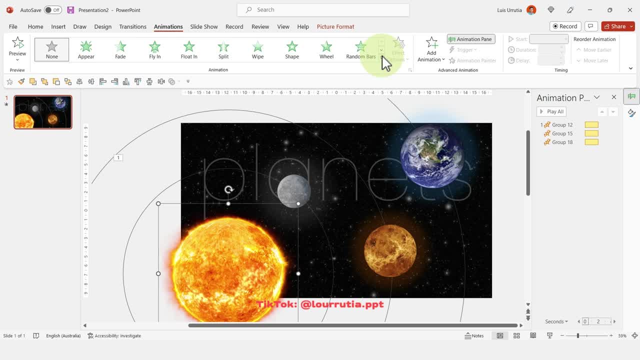 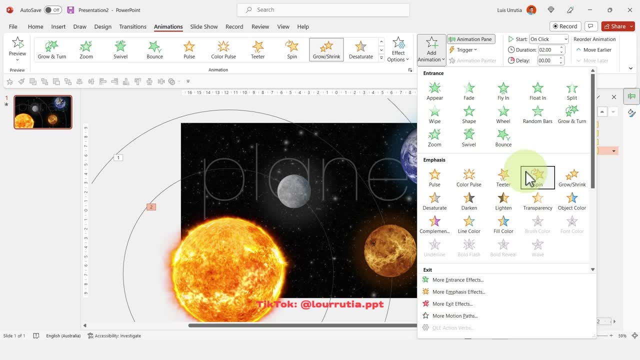 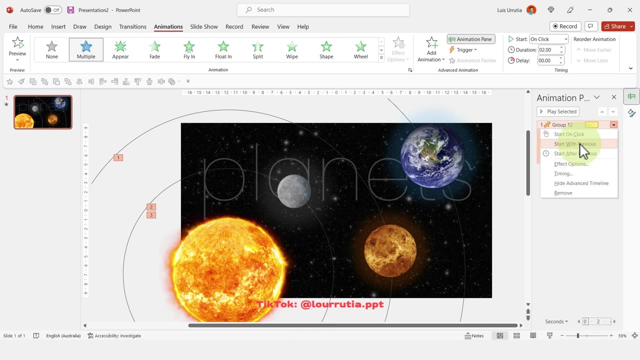 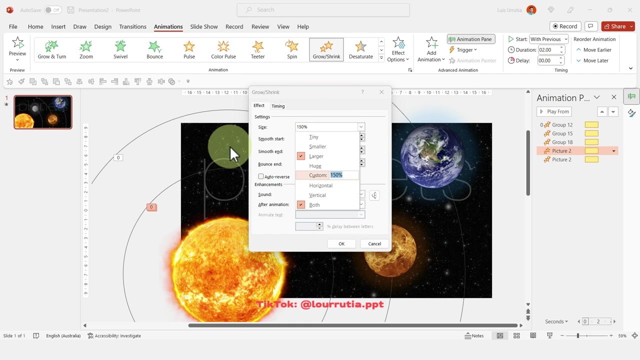 and for the animation of the Sun. first I go to and me animations, click on grow and shrink, then go to add animation and select spin from the animation pane. you can right click and start with previous so the animation starts automatically. and then, if you right click and go to the effect options here for the grow and shrink effect, I'm gonna 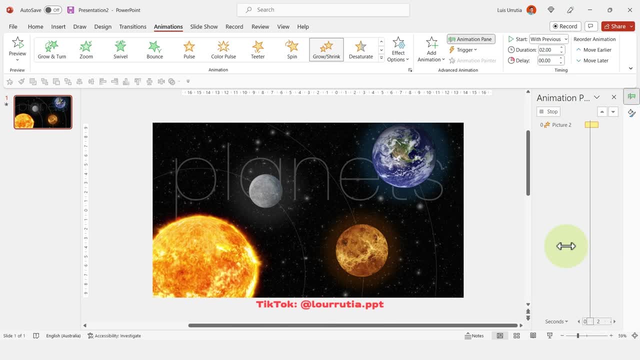 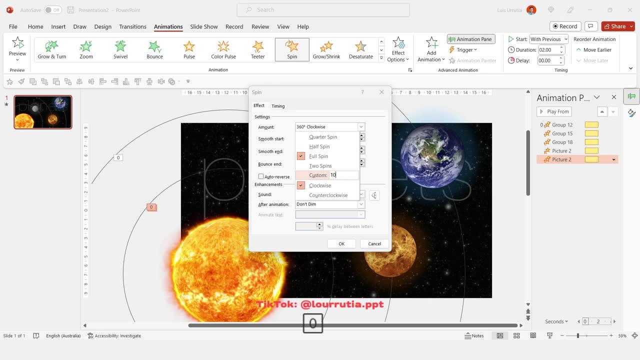 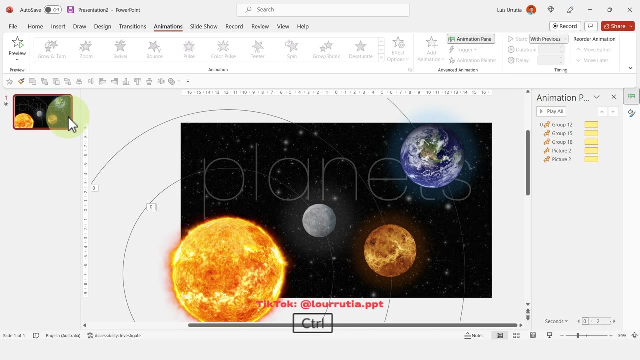 change it to 105, because I want it to be very subtle and for the spin animation, instead of having 360 degrees, I'm gonna change it to 10. so now, when I click play, all I just get like this very subtle effect, which is super, super cool. so then you duplicate the slide with ctrl d and for. 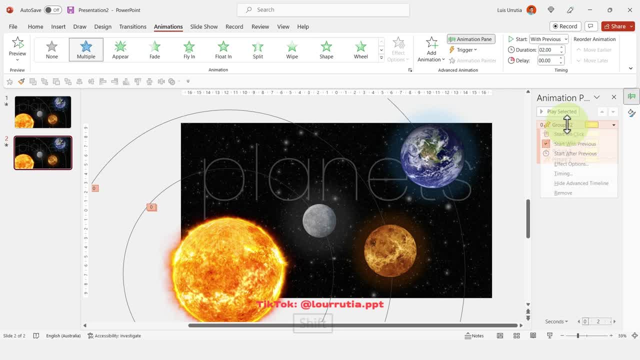 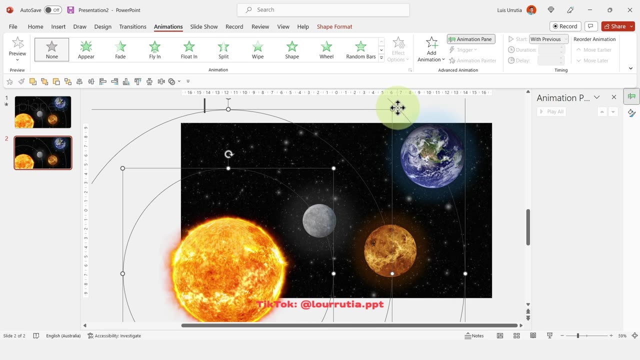 the morph transition to work, we need to get rid of the animations here. so select the animations from the animation pane, right click and remove, and then I'm gonna push up the word planets and then I'm gonna select the the, the orbits here, and I'm gonna make them transparent from the format object panel. so here you click. 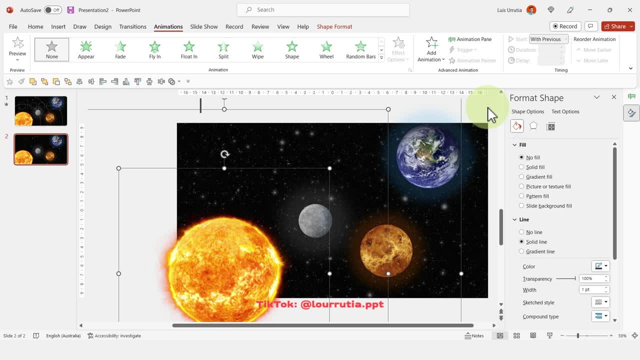 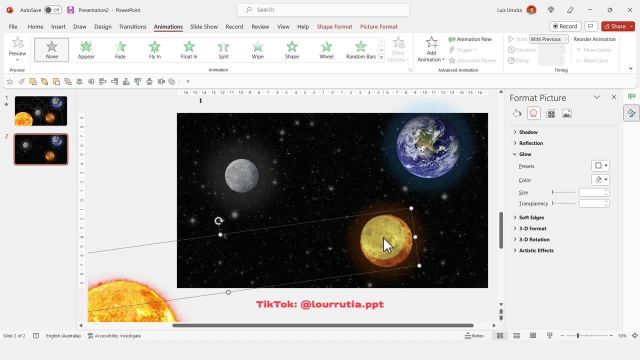 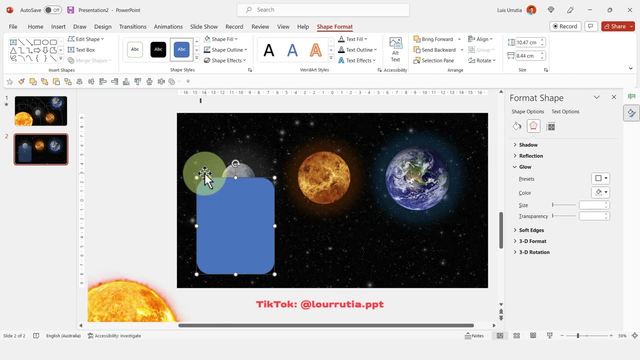 online and then change the transparency to 100 and then we're gonna move this sun to the left, to the gray area of the slide, and then we're gonna position the planets here in a row and then I'm gonna insert a rounded rectangle here. remember, with the yellow dot here you can change the. 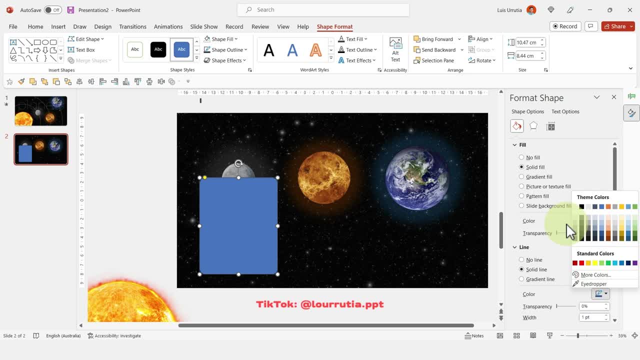 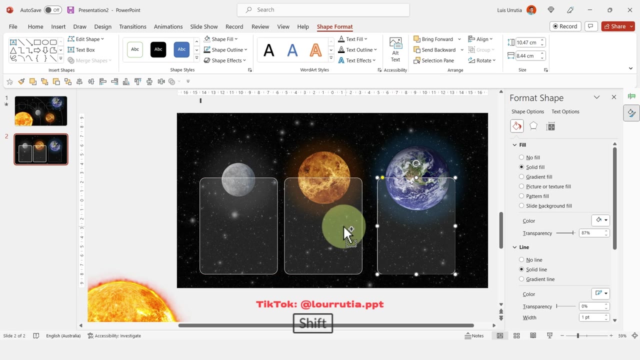 roundness of the corners and then click on solid line, select the white line, and on fill, select a white fill and just change the transparency a little bit so we can see through the shape, and then you can duplicate it a couple of times with holding ctrl on your keyboard and dragging your 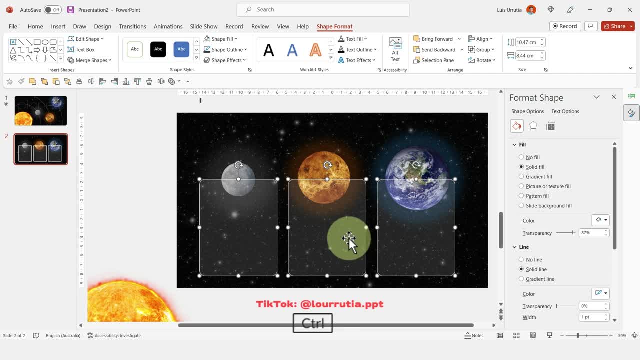 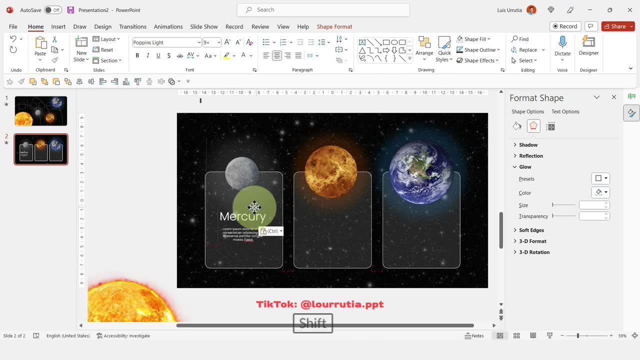 mouse you can distribute them horizontally with the aligned panel, and then you just select the planets, right click and then you can duplicate them horizontally with the aligned panel and then you can bring to front. and then I just added some text. I added the the name of the planet, a little. 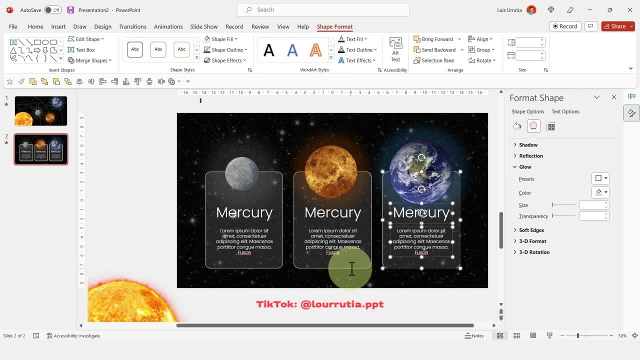 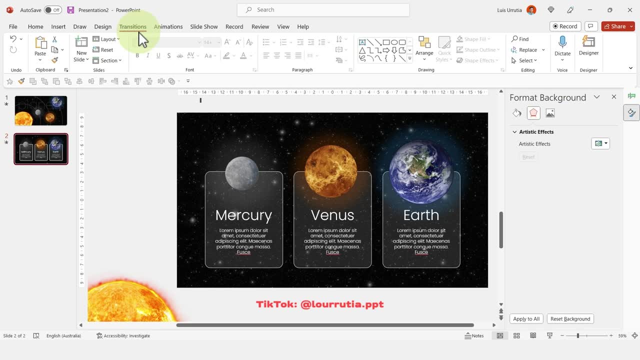 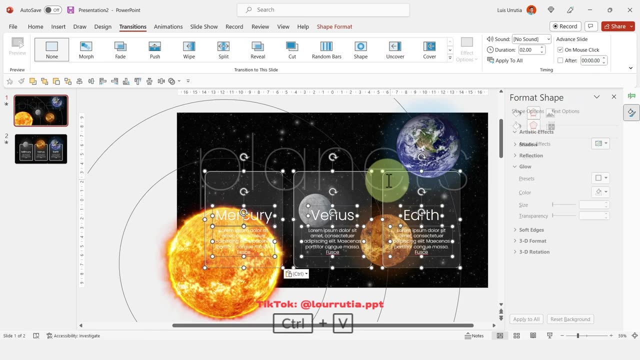 description maybe, and overall something just like very basic. and while I'm doing this, please don't forget to follow me on instagram at lurutia ppt. and then we're gonna select these new shapes that we did, so that means the texts and the shapes, and we're gonna copy paste them on the first slide and 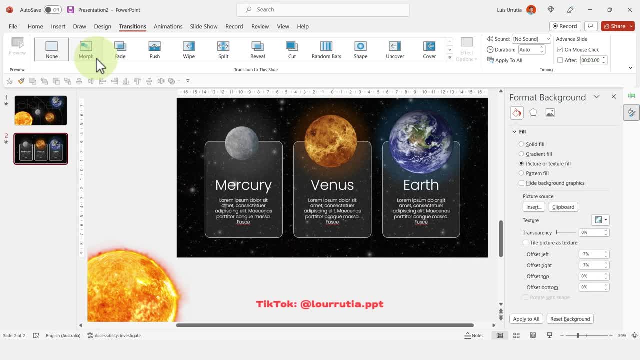 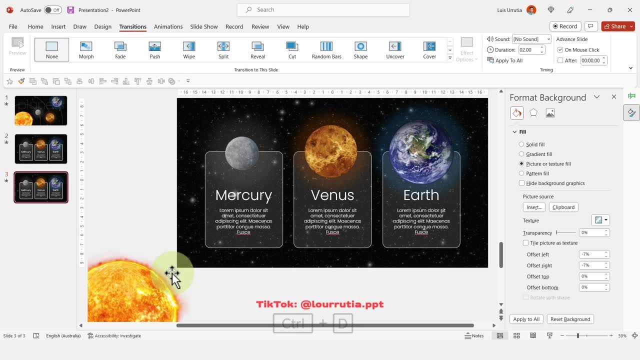 drag them to the next slide, and then we're gonna copy paste them on the first slide and drag them down to the gray area, right click, send to back. so now, if we apply the morph transition, we're gonna get a very cool effect. and now we're gonna duplicate that slide with ctrl d and we're gonna 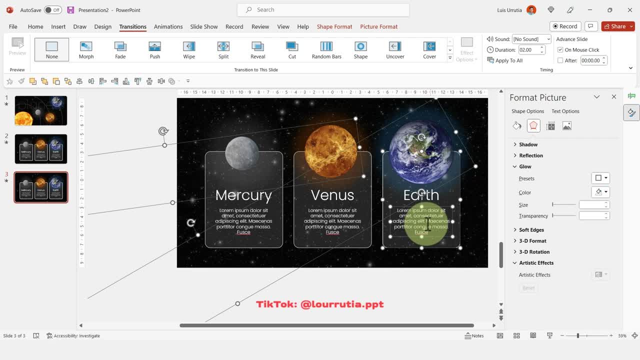 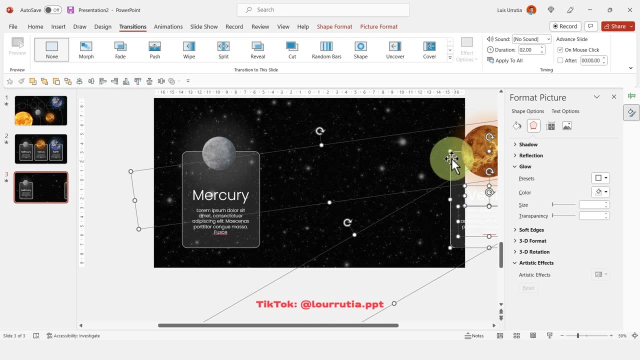 delete the sun, and then we're gonna select the venus and earth, because we're gonna focus on mercury. so we select everything related to those planets and we're gonna drag them out of the composition to the right- and now I'm gonna make this container a little bit larger- and then we're 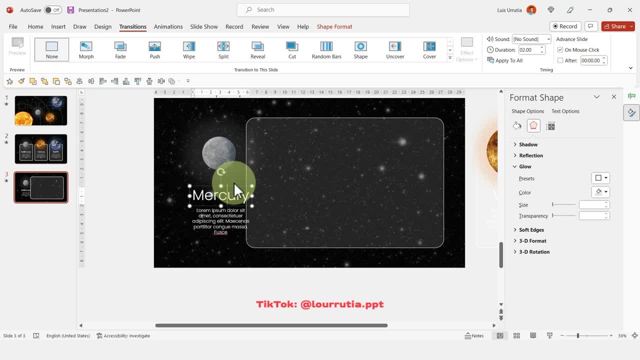 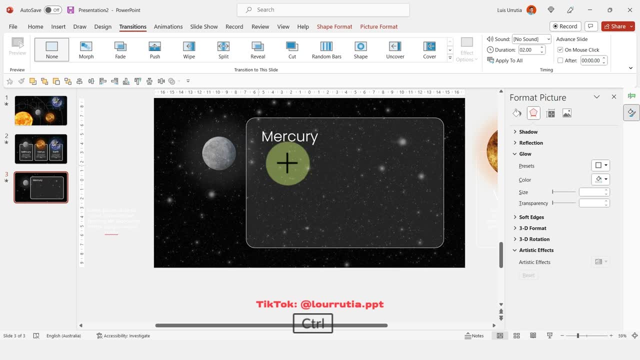 gonna move it to the center, because that's where our information about this planet is gonna. it's gonna go, and then I'll move the title here and the description out of the composition and then select your planet and make it bigger, holding shift in your keyboard, and then I'll insert a. 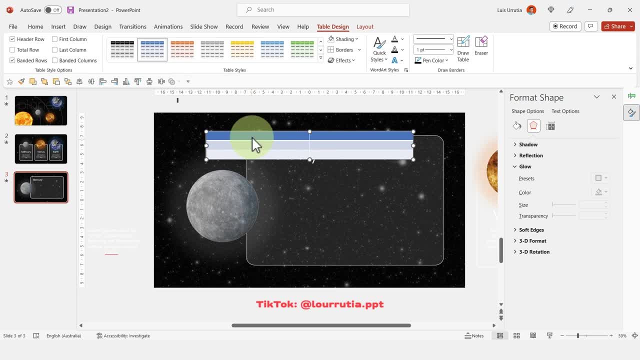 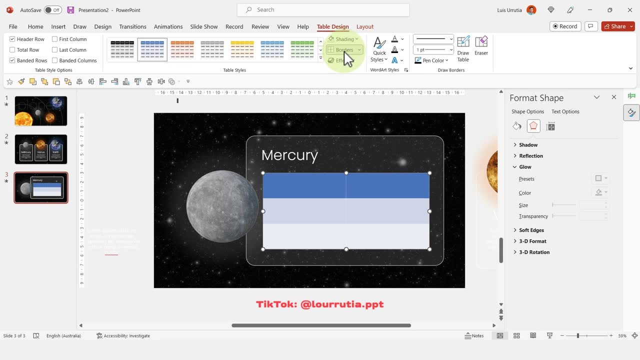 table. so this one will be two by three and I'm gonna get rid of the borders and I'm gonna get rid of the shading as well. so I go here, select no borders, and then I'm gonna move this to the no field for the shading. now change the pen color here to white and select the inner border. so